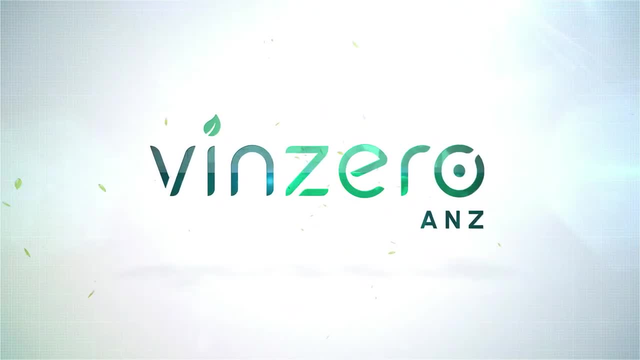 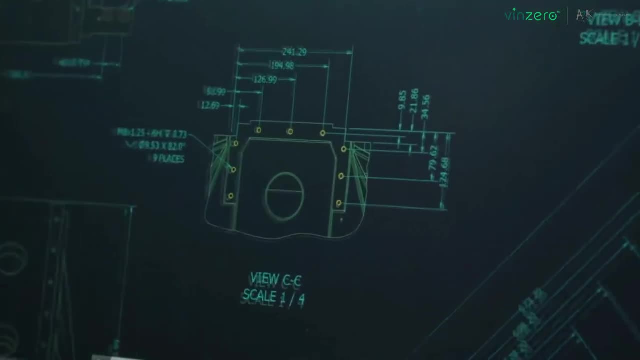 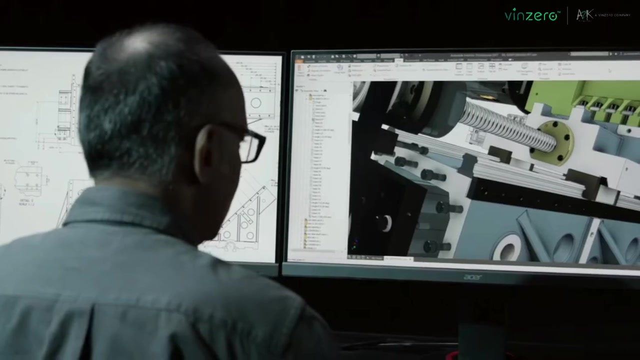 What is 3D modelling? 3D modelling is the process of using computer-aided design software to develop a virtual mathematical representation or design of a desired object or part. 3D modelling can either result in a digital or physical end product. The digital 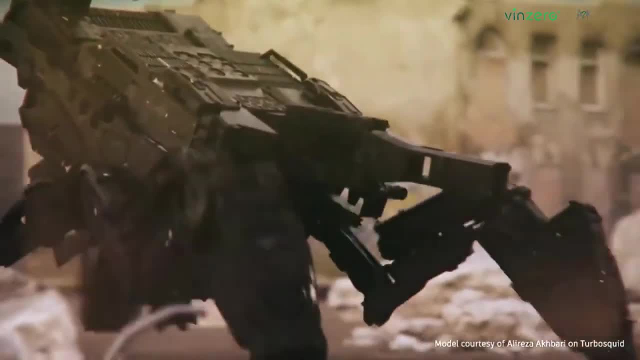 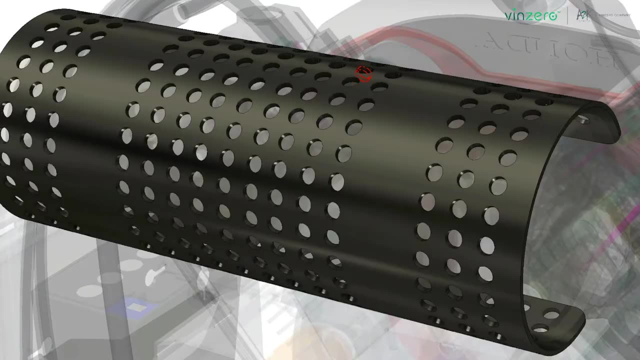 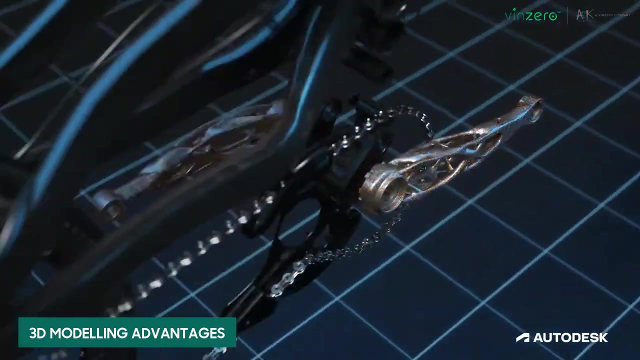 animation and film industries both use 3D modelling to bring storytelling to life on your screen. Industrial designers and engineers, however, use 3D modelling to create a digital representation of products they intend to manufacture in real life. 3D modelling advantages. 3D modelling offers significant advantages over 2D drawings when 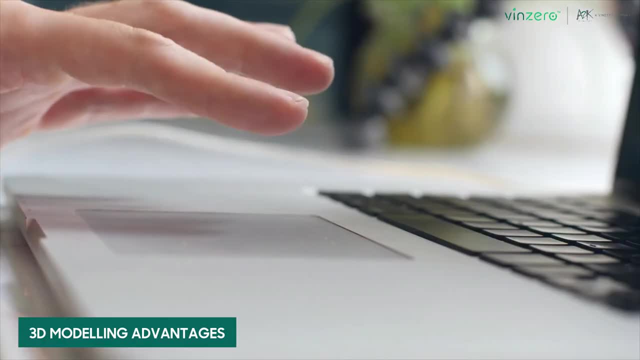 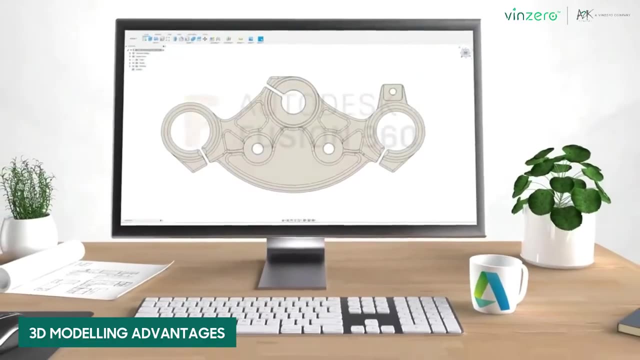 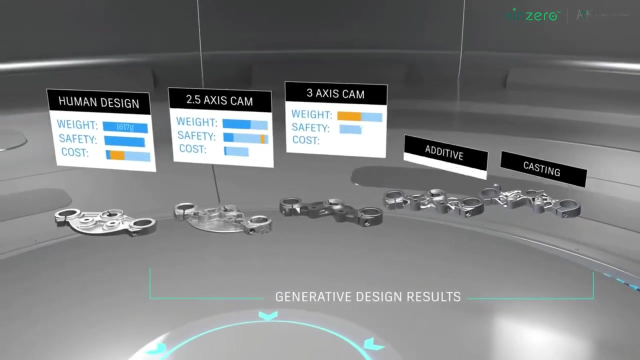 using the right design software Within CAD software, designers can create 3D models by manipulating virtual space. Modern CAD software like Autodesk Fusion 360 provides additional aids like generative design, An artificial intelligence or AI-driven predictive method that calculates thousands of feasible. 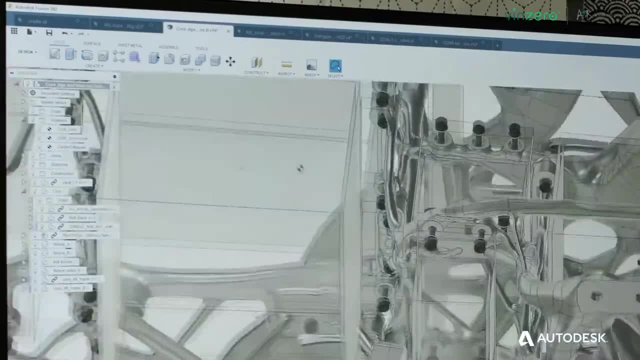 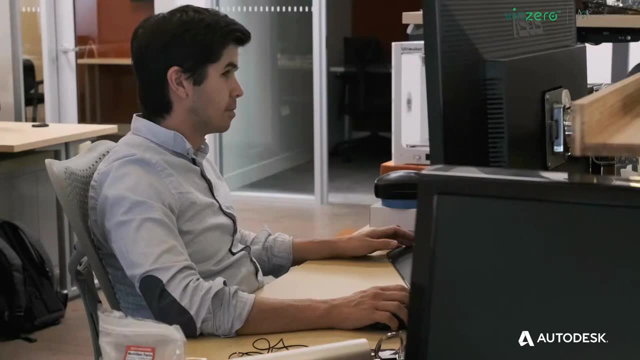 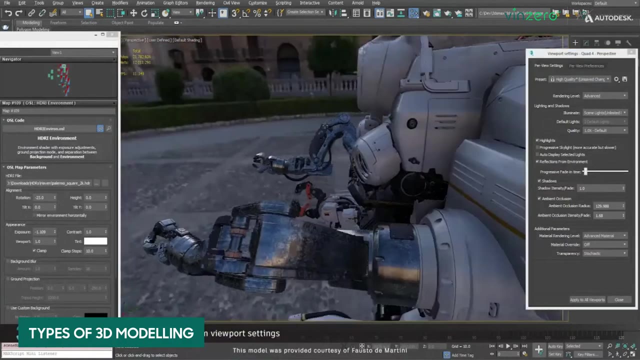 3D models. 3D models live in a digital environment. With the proper CAD software, designers and engineers can manipulate, test and revise their designs to find the ideal balance between form, function, durability and aesthetic appeal. Types of 3D modelling: There are two general types of 3D modelling. 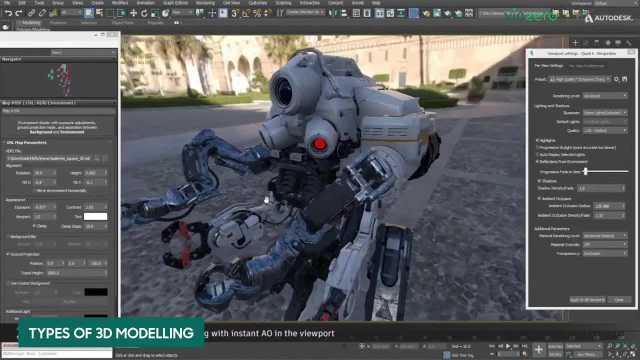 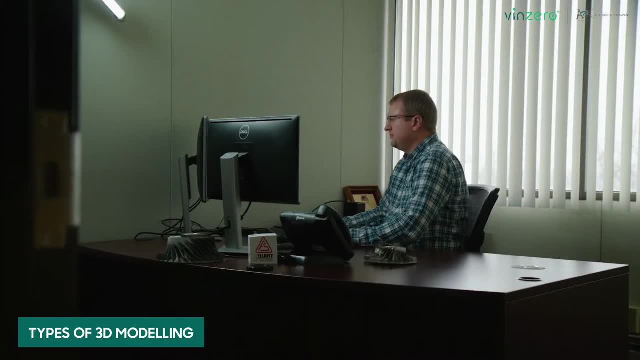 – organic and hard surface. Organic modelling is generally the digital 3D modelling. Organic modelling is generally the digital 3D modelling. Organic modelling is generally the digital recreation of organic or living things like trees, animals and people. Often organic modelling also incorporates animation. Hard surface modelling deals with inorganic materials. 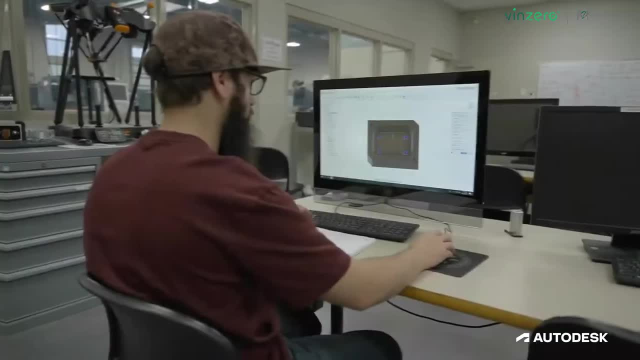 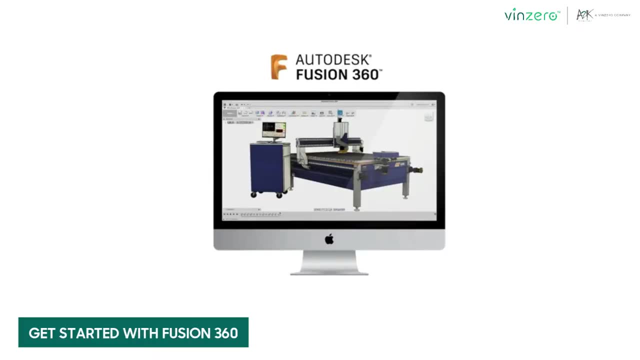 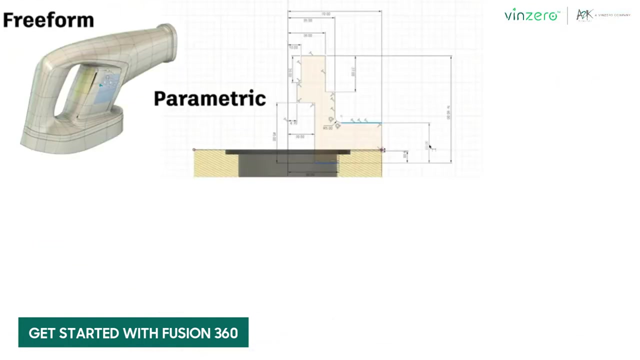 and static objects such as machine parts, automobiles or furniture. This is the type of modelling most pertinent to industrial engineers. Get started with Fusion 360 3D modelling software for beginners. Fusion 360 is an integrated cloud CAD solution that also provides computer-aided manufacturing. 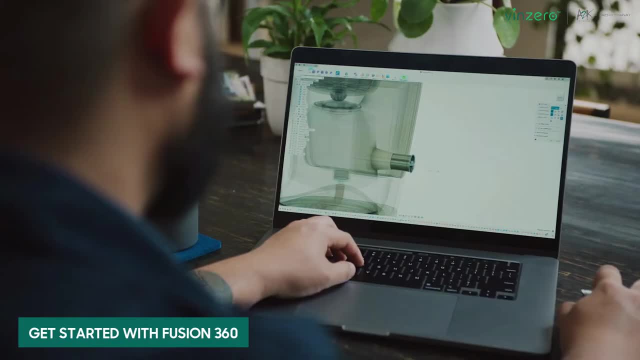 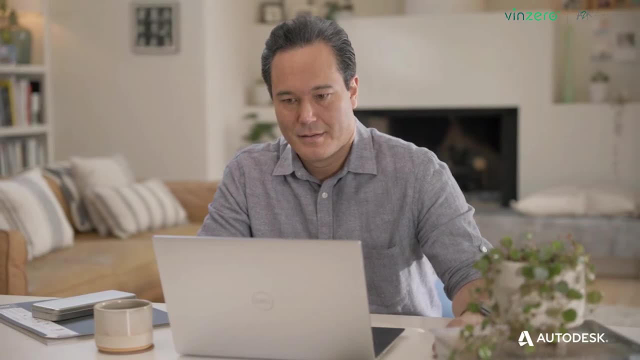 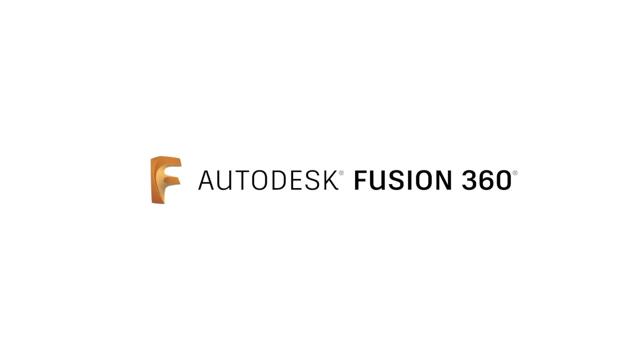 computer-aided engineering and printed circuit board solutions. Fusion 360 is user-friendly and provides some of the most comprehensive training materials on the Internet for beginners. Streamline your design workflow and consider Fusion 360 for your next 3D modelling project. Contact us today in the description below for more information.